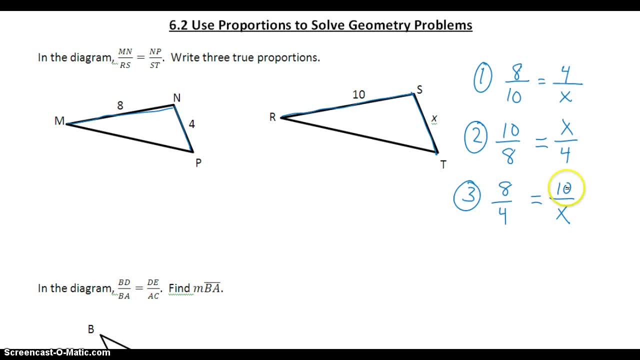 proportion. in my numerator 8 and 10, I've kept this ratio And in my denominator 4 and X, I've kept this ratio. 8 to 4, 10 to X. This proportion is equal to 10 to X. 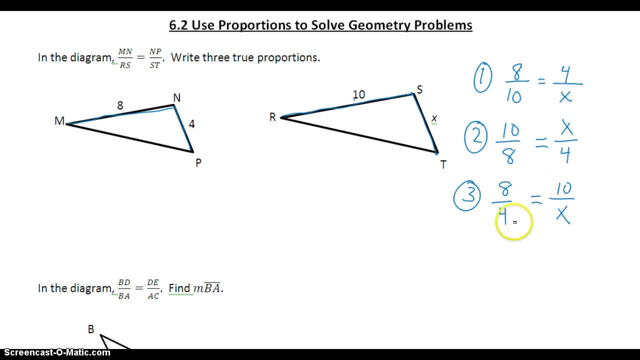 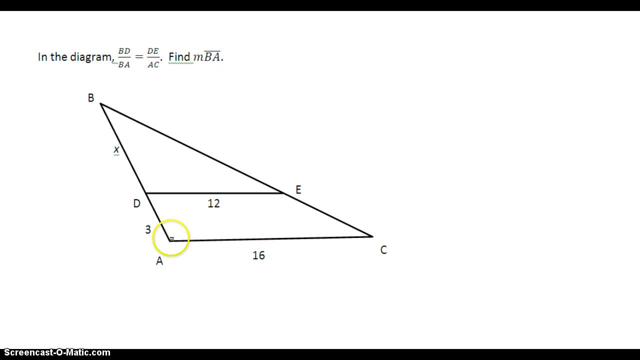 This proportion is also equivalent. It's also true. Let's use that concept to solve for a missing length. I need to find BA. Well, in order to find BA, I'm going to first find BDX, So I'm going to redraw these two triangles. 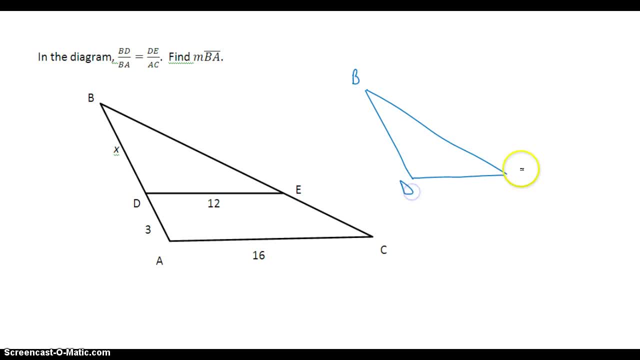 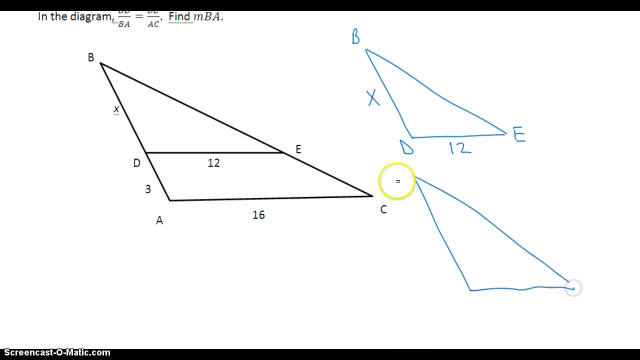 I have a small triangle, BDX. I have a triangle BD and E, where my side lengths are X and 12.. I also have a larger triangle, BAC. AC has a length of 16.. And BA has a length of X and 16.. 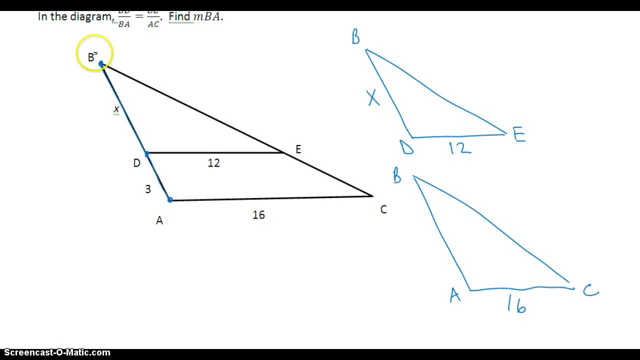 So I want to make sure I write BA as X plus 3.. A lot of students mistakenly will write this as 3X. I don't want to multiply these two lengths, I want to add them. So if I look at my directions I can set up a proportion. 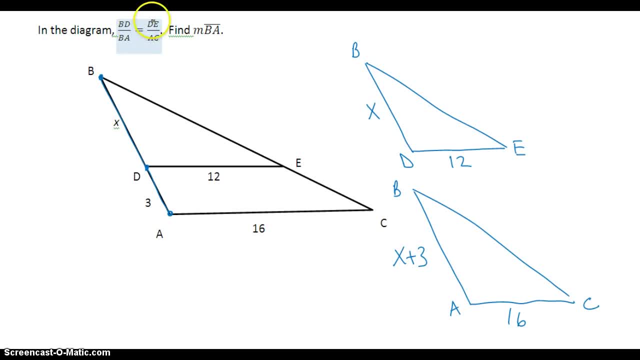 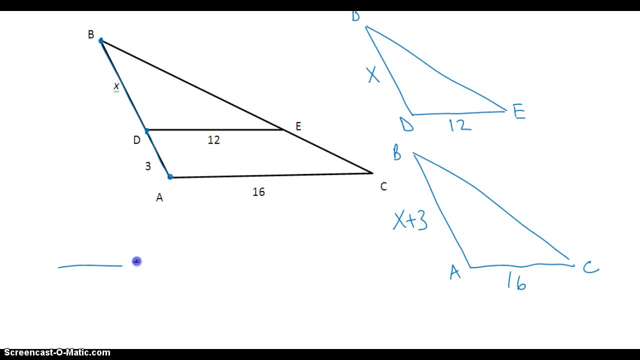 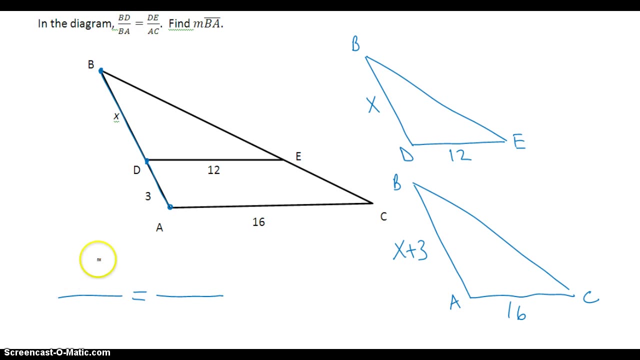 BD over BA equals DE over AC. So I'm going to do that math, I'm going to set up my proportion where I have BD, which is X, over BA, which is X plus 3.. DE, which is 12, over AC, which is 16.. 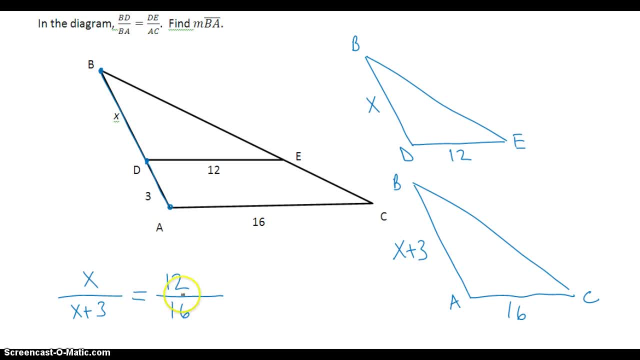 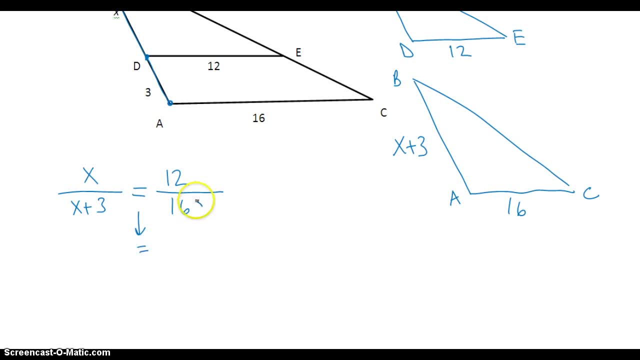 At this point I have a proportion with an equal sign I can solve. I can drop my equal sign straight down And cross multiply 16X equals 12 times X plus 3.. Notice that X plus 3 gets put into parentheses even though it didn't have parentheses here. 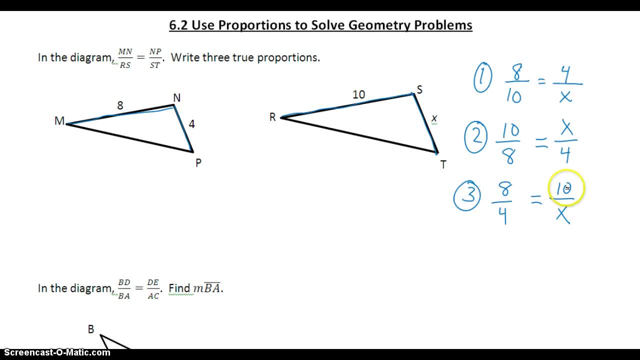 proportion. in my numerator 8 and 10, I've kept this ratio And in my denominator 4 and X, I've kept this ratio. 8 to 4, 10 to X. This proportion is equal to 10 to X. 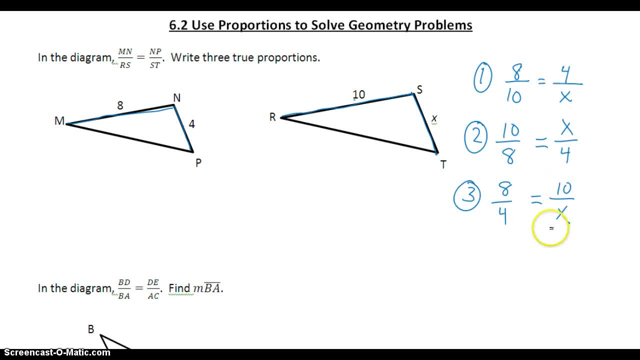 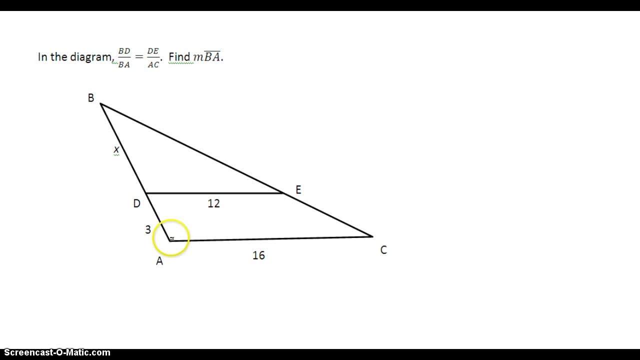 This is also equivalent. It's also true. Let's use that concept to solve for a missing length. I need to find BA. Well, in order to find BA, I'm going to first find BDX. So I'm going to redraw these two triangles. I have a small triangle, BDX. I'm going to 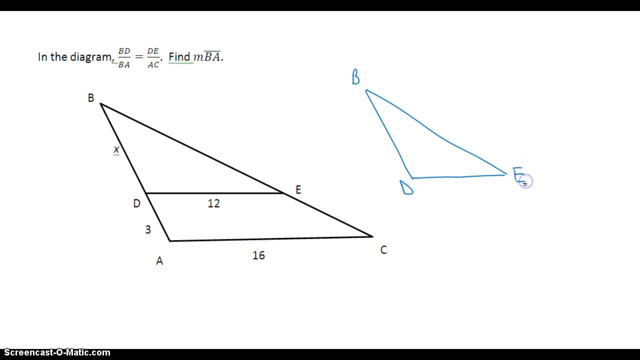 leave this one at my original value. I also have a big triangle. BDD where I have x is equal to 12: 2. In the middle of my side of triangle and this will be products Center, I'll have this side language, If I can just decrease a little bit ofściple to help with. 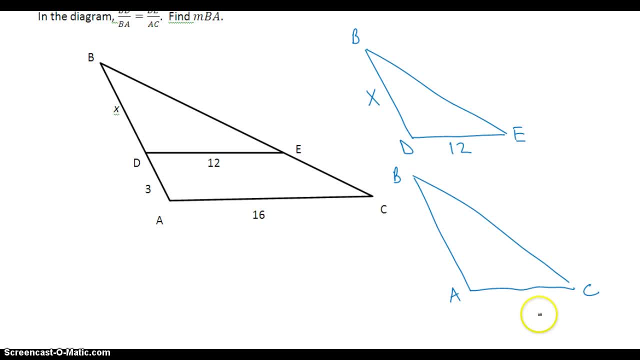 Initially bound and then sort it out. for example, if I look at the x axis, I can just cut it around this way. In this case, I'm going to say these two triangles, BD and E, which are x and 12. And I also have a larger triangle, BAC. So these three sideᅠs have a length of 16, and BAC has a length of X-u and 3.. 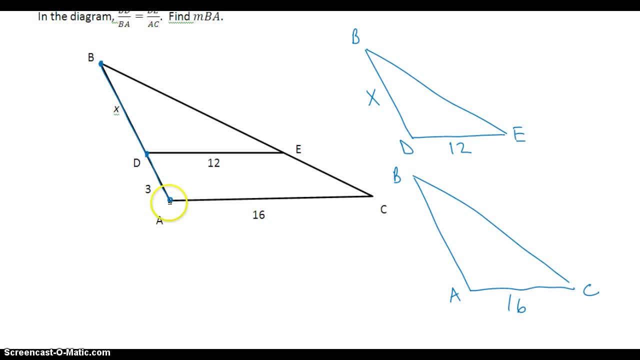 I need also to write this triangle with the these three times this information I need And if this triangle is true, then this card product will be somewhat more correct and spin-free: 3.. So I want to make sure I write BA as X plus 3.. A lot of students mistakenly will write this as: 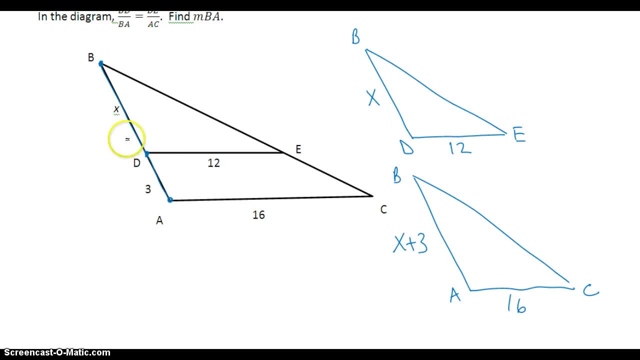 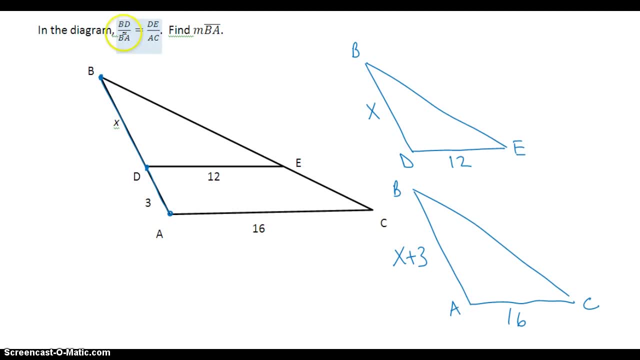 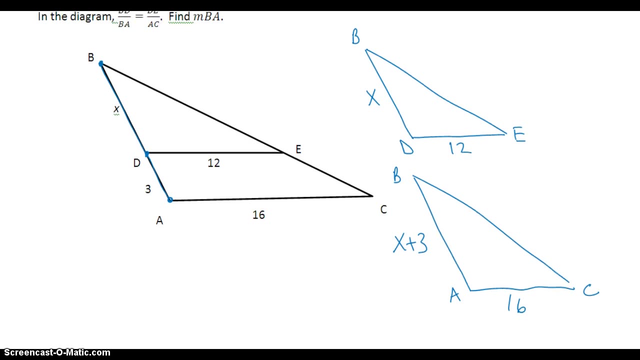 3X. I don't want to multiply these two lengths, I want to add them. So if I look at my directions, I can set up a proportion. BD over BA equals DE over AC. So I'm going to do that math, I'm going to set up my proportion. 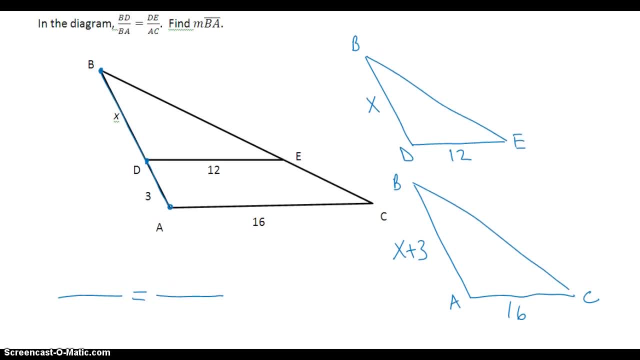 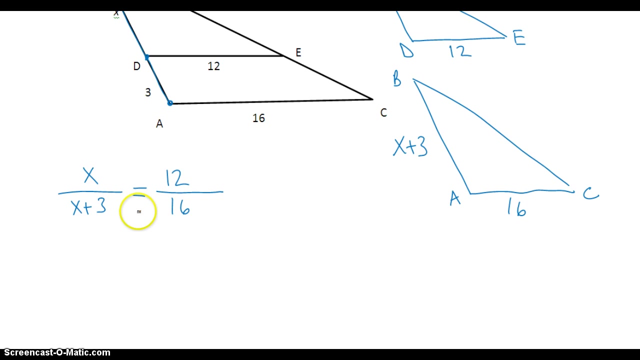 where I have BD, which is X, over BA, which is X, plus 3, DE, which is 12, over AC, which is 16.. At this point I have a proportion with an equal sign I can solve. I can drop my equal sign straight down and cross multiply.